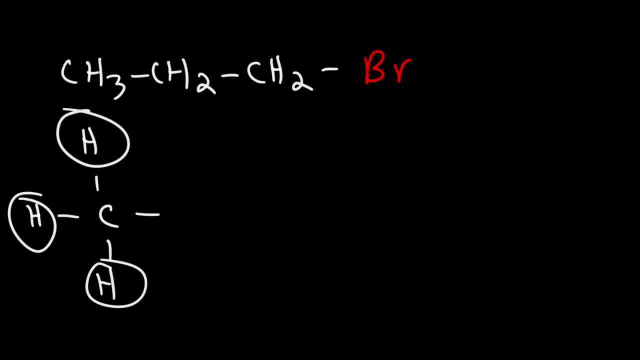 exact chemical environment. They are all attached to the same carbon atom and they're all adjacent to each other, To this group. So those three hydrogen atoms are chemically equivalent, which means that in an HNMR spectrum they will show up as just one signal. So generally, 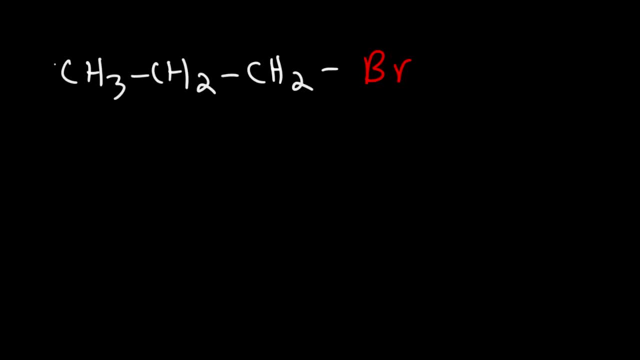 speaking, the hydrogen atoms that are attached to a particular carbon atom usually show up as one signal- Not always, but usually- So we can call this signal A to correspond to those three hydrogen atoms. Now, these two hydrogen atoms are in a different chemical environment than these. 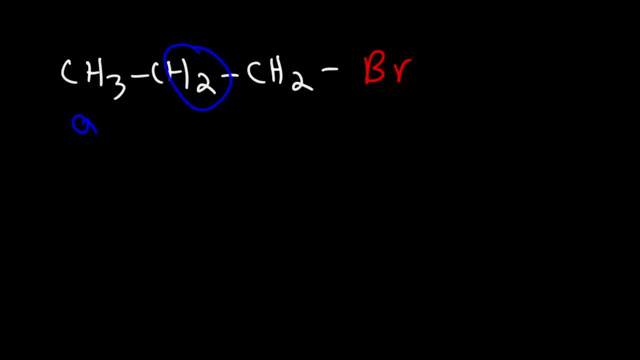 three, because they're closer to the bromine atom. So they're going to show up as a different signal. And these two hydrogen atoms in the CH2, they're closest to the bromine atom. In fact they're attached to the same carbon atom. 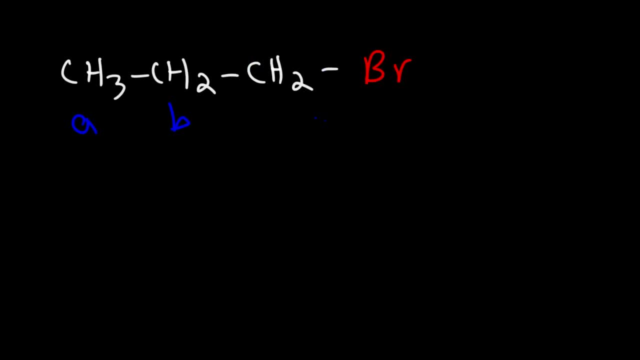 as the bromine atom. So they're going to show up as a different signal compared to the other hydrogen atoms. So for this particular molecule we're going to show up as a different signal. So for this particular molecule we should expect three signals in the HNMR. 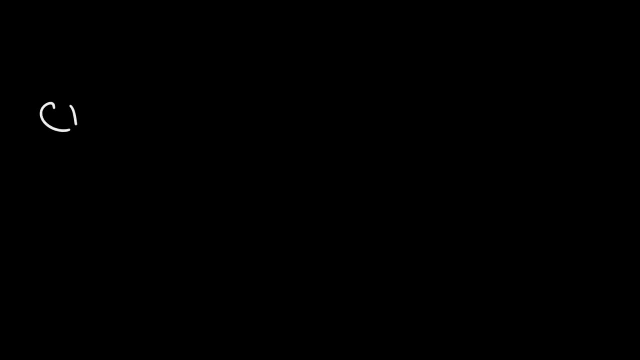 spectrum. Now let's try another example. Let's say: if we have a molecule of propane, How many different signals would you expect to get from an HNMR spectrum in this molecule? Now, what I like to do is draw a line of symmetry. 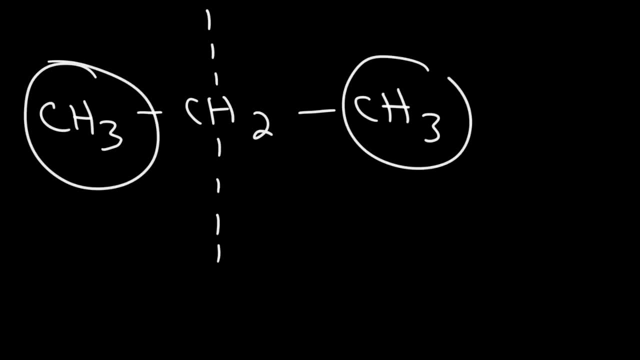 Notice that the left side looks like the right side When you see that this tells us that the hydrogens in the methyl groups on the left and right are equivalent. They're in the same chemical environment. Now the CH2 hydrogens are different than the CH3 hydrogens, so we can call this signal B. So for this, 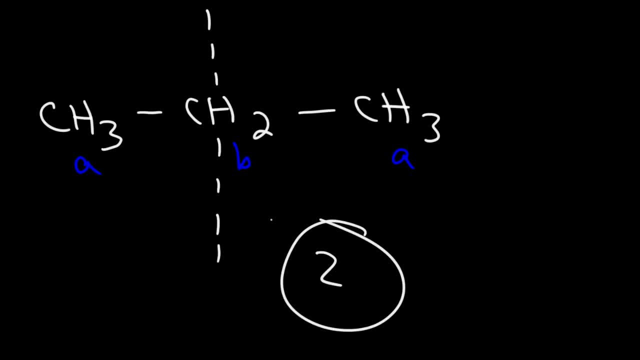 particular example, we should expect two different signals in the HNMR spectrum. What about this example, Dimethyl ether? Once again, we can draw a line of symmetry in the middle, and so the methyl group on the left is identical to the. 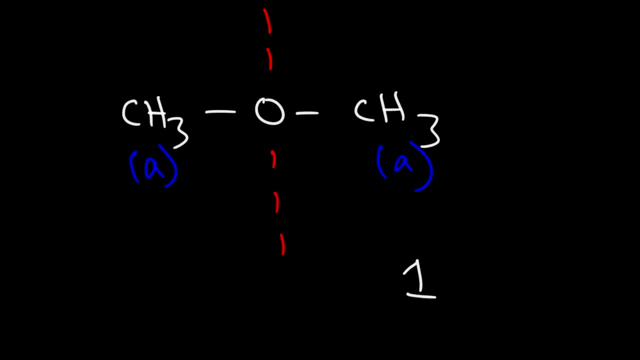 methyl group on the right. So in this case we are only going to get one signal for that molecule. Try this one. So how many signals should we get for this molecule? The first thing I like to do is identify the hydrogen atoms that are identical to 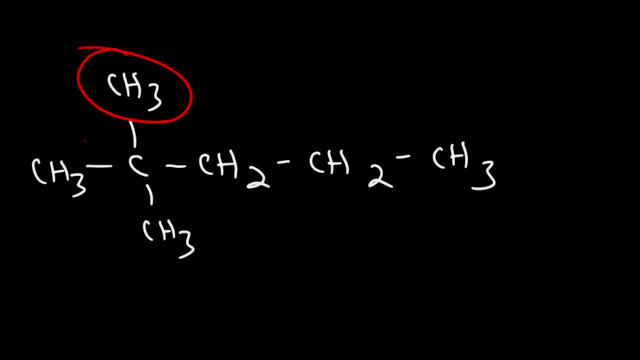 each other. So, looking at these three methyl groups, they are attached to the same carbon atom and, due to the free rotation of carbon-carbon single bonds, they are equally close to this group. Therefore, those three signals, well, those three methyl groups- will show up as one signal, So we can call it signal A. They 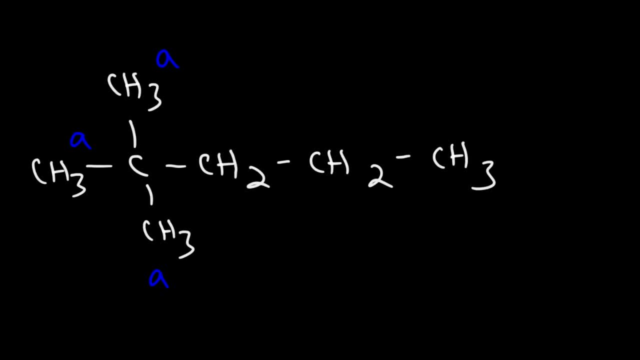 have the exact same chemical environment. Everything else is going to be different. This is going to be signal B, C and D. As you can see, these two CH2 groups, they're not the same. they don't have the same chemical environment. This one is close to the. 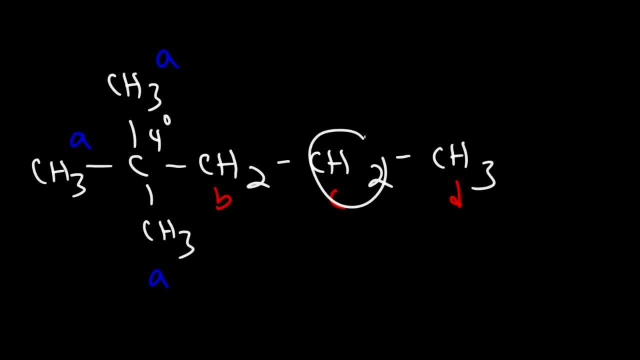 quaternary carbon, and this one is further away, but it's adjacent to the methyl group. This one is not adjacent to the methyl group, so they're different. Thus we should have a total of four different signals. Now let's start. 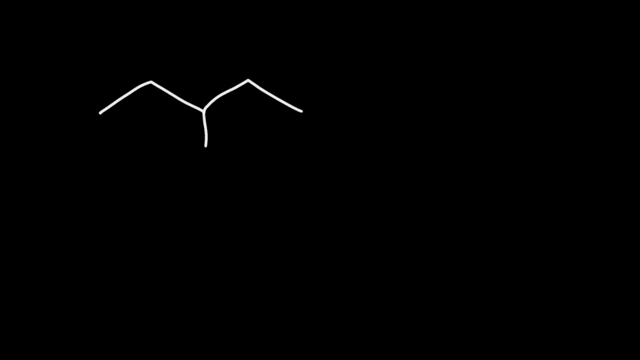 using line structures in our examples. So let's say we have three bromine pentane, How many different signals should we get in this molecule? So we could say that the line of symmetry is at the third carbon and we can call this signal A. 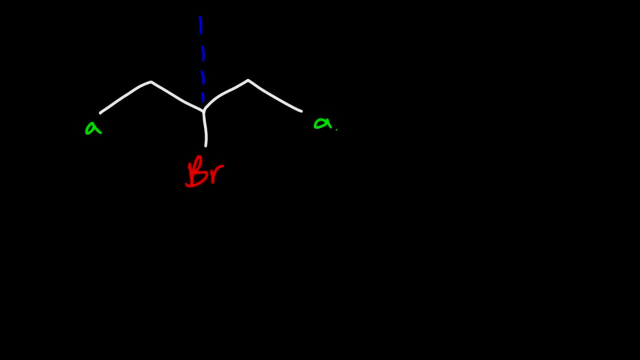 because they're equidistant from the line of symmetry, and the hydrogen atoms attached to those carbons. that's going to be signal B, and there's one hydrogen atom attached to this carbon which will correspond to signal C. So this particular 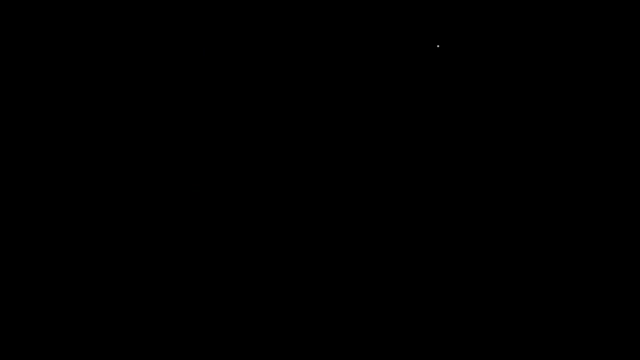 molecule is going to have three signals. Try this one: 2-methylpentane. How many different signals should we get in this case? So here we have two methyl groups attached to this carbon, so those two methyl groups will be identical to each other. so that's going to be signal A. We do 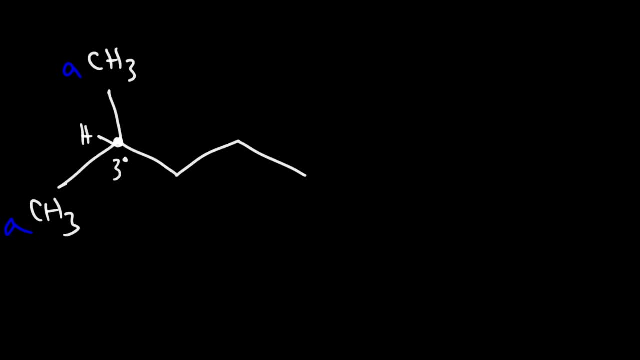 have a hydrogen atom attached to this tertiary carbon, so that's going to be signal B and then the rest are different. We really don't have a line of symmetry in this case, so all the other hydrogen atoms on the different carbon atoms will. 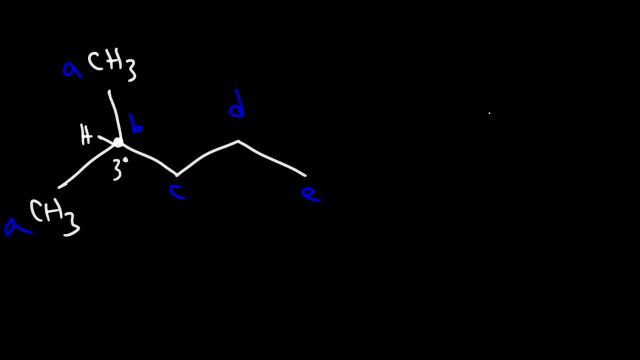 be different at the right side. Thus we have a total of five signals for that molecule. Here's another one that we can work on. Try that one. So for this particular example, I'm going to draw the line of symmetry here, since we have a. 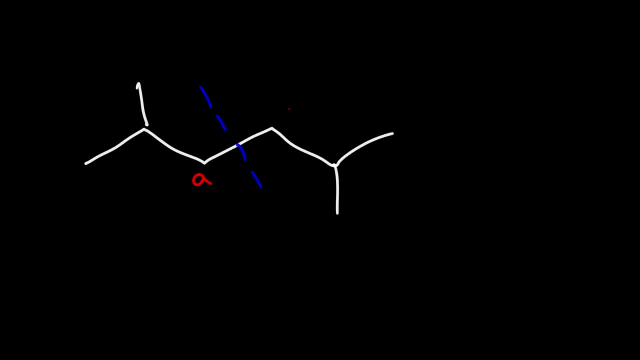 symmetrical molecule. Now the hydrogen atoms on those two carbon atoms, they're equidistant from that line of symmetry, so they're going to be identical. and then these two hydrogen atoms corresponding to signal B, they will be identical. Now what about the methyl groups? 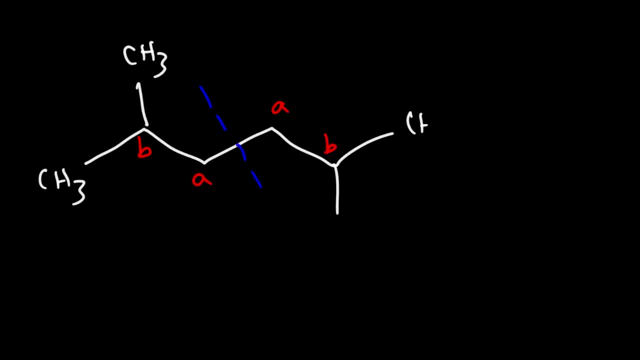 Now, what about the methyl groups? Now, what about the methyl groups? Are they identical to each other? Should we say this would be signal C and this would be signal D, or are all four of them identical to each other? It's important to understand that these two are definitely identical to each. 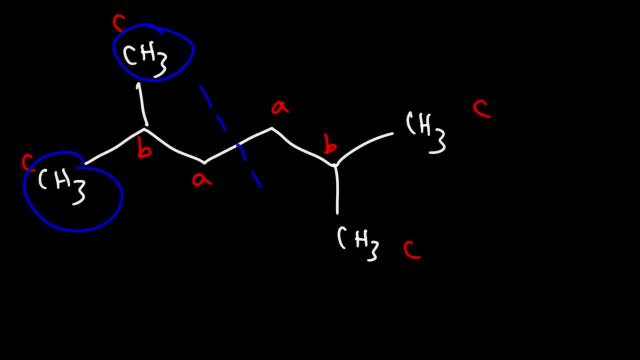 other, because we've covered examples like that before, But also these two are identical to each other. They're equidistant from that line of symmetry. They have the same exact chemical environment, and so thus all four of them are identical to each. 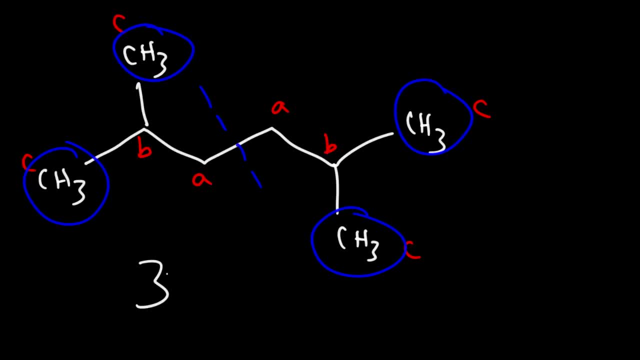 other. So, for this particular situation, we have a total of three different signals in the H-NMR spectrum. Now, what about this one? Now I'm going to ask you two questions: How many signals should we get in the H-NMR spectrum and how many? 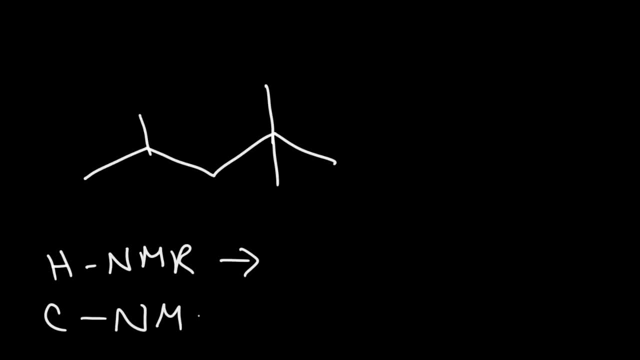 should we get in the CMMR spectrum? So let's focus on hydrogen. Now. we don't have a symmetrical molecule, so there's really no line of symmetry. Nevertheless, these three methyl groups are identical to each other, So in the HMR spectrum, 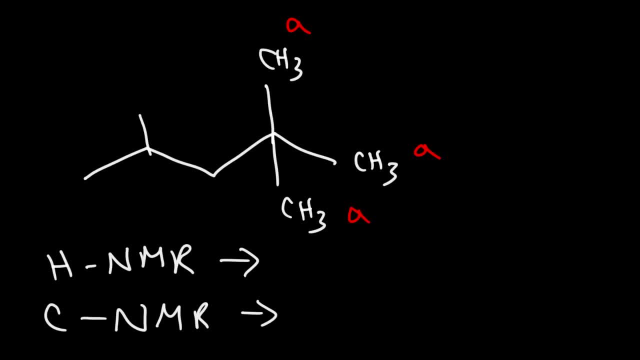 they will show up as signal A. Now these two methyl groups are identical to each other, so they will show up as signal B. Now we have a hydrogen atom on the tertiary carbon, so that's going to be signal C, and this is a CH2 group. so 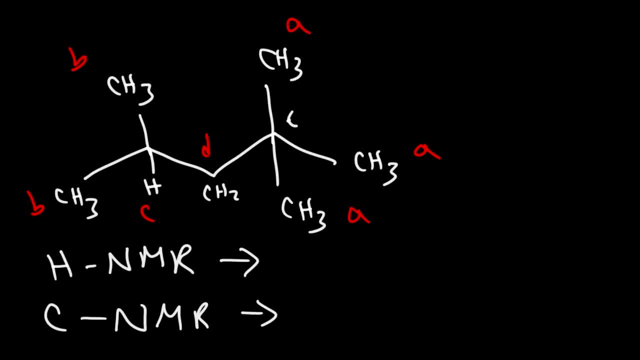 that's going to be signal D. Now this particular carbon has no hydrogen atoms, so in the HMR spectrum we should only get four signals. Now we do have a carbon atom here, so I'm going to use a different color for the CMMR spectrum. 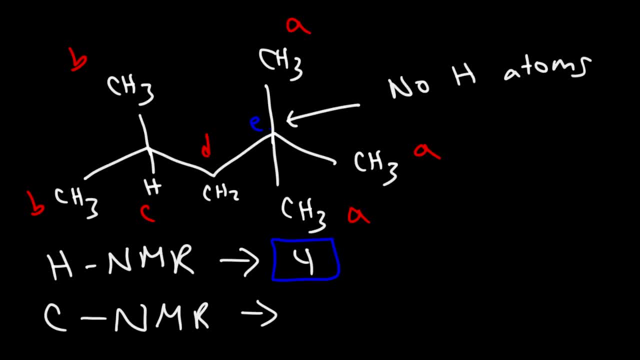 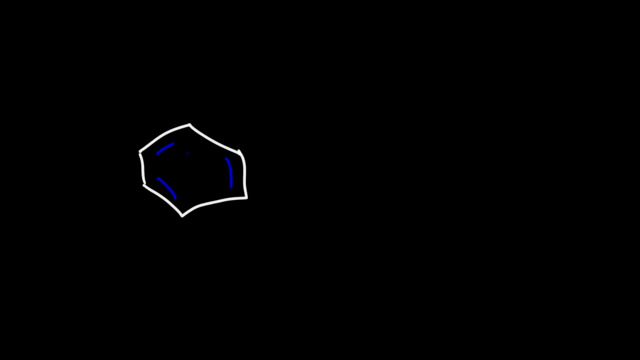 that's going to be basically signal E. So we should have a total of five signals in the carbon 13 NMR spectrum. Now for the next example. we're going to use a benzene, So how many signals should we get in the HMR spectrum? 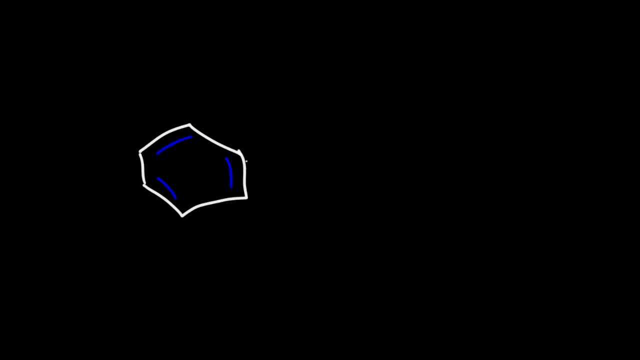 Now it's important to understand that every carbon atom in benzene has one hydrogen atom, and all six of these hydrogen atoms are equivalent to each other. They have the same chemical environment. so this will show up as one signal. Now let's change it up a bit. 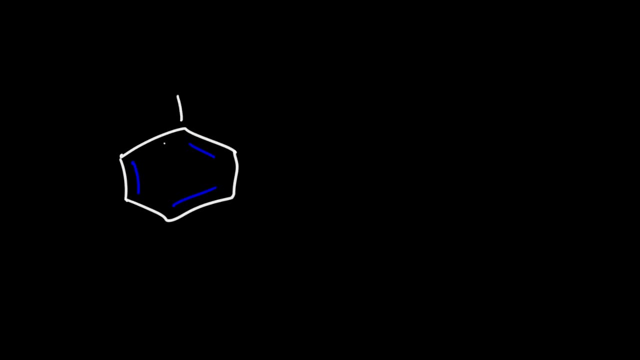 So instead of benzene, let's say we have bromo benzene. How many different signals should we get in h Kit于we spectrum? Also, what about the carbon-13 NMR spectrum? So, focusing on hydrogen, this will be signal A. We could draw the line of symmetry. 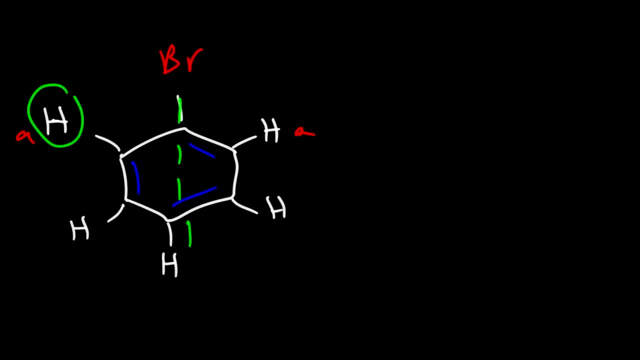 right at the center, These two hydrogens. they're one carbon away from the bromine atom, so they have the same chemical environment. This would be signal B. They're two units away from the carbon with the bromine atom, And this one is three units away. so that's going to be. 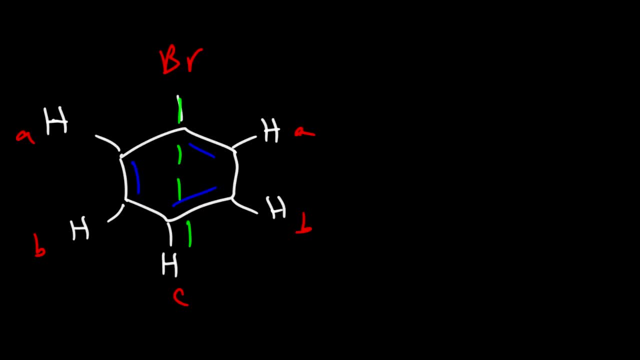 signal C. Now let's focus on the carbon-13 spectrum. So the carbon atoms here are identical, just as the hydrogen atoms on them are identical. Now, these carbon atoms, they will correspond to signal B. They're identical too, And this one is different. Now we do have a carbon atom here. 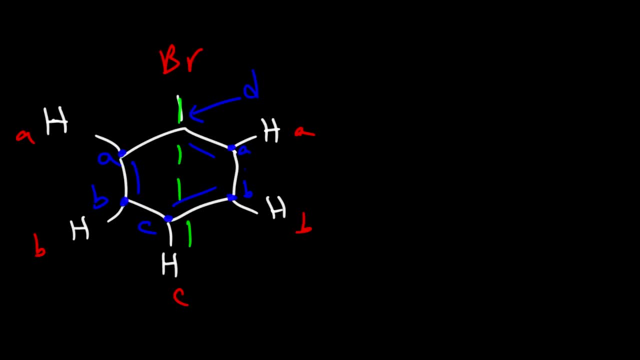 but it doesn't have a hydrogen atom, So that will show up as the fourth signal in D In C NMR. So in the H NMR spectrum we have three different signals indicated using the red color And in blue. for C NMR we're going to have a total of four signals. 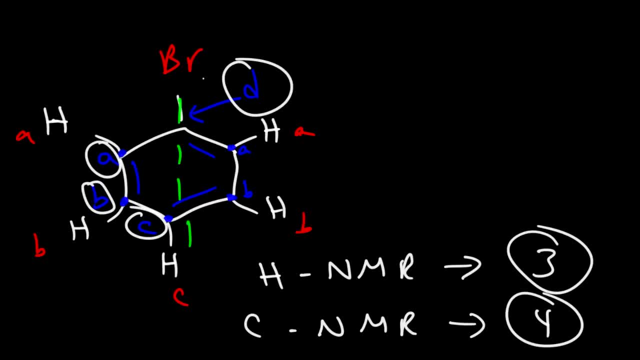 A, B, C and D. So be careful if you're dealing with C NMR or H NMR. If you have a test, make sure you pay attention to this because it can affect the carbon-13 spectrum. So if you have a test, make sure you pay attention to this. 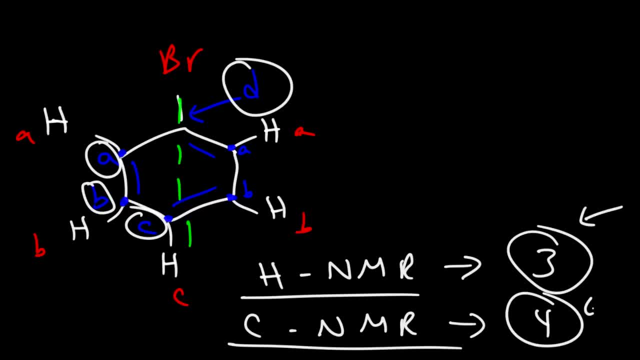 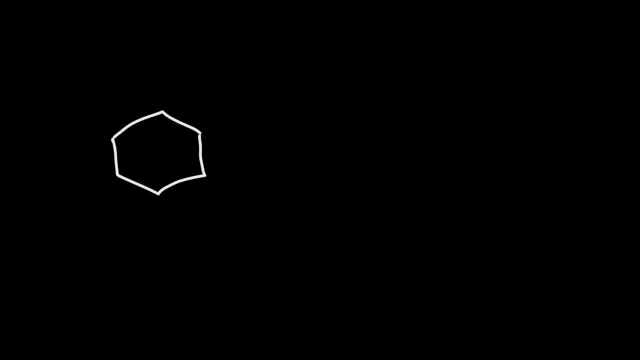 it can affect your answer. As you can see, the number of signals for these two different spectrums can be different. Now let's work on para-xylene as an example, And we're going to focus on both H NMR and C NMR. So how many H NMR signals should we get for this? 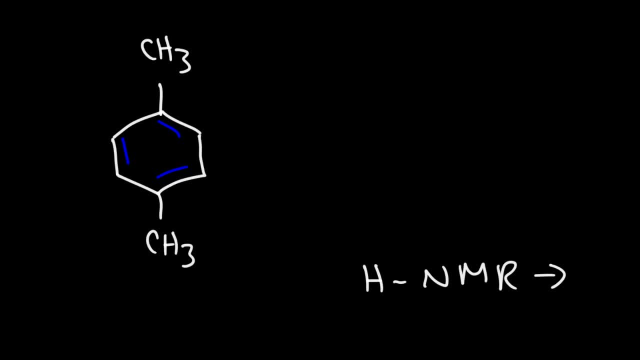 molecule. So let's identify all of the hydrogen atoms first, And let's also identify the line of symmetry which is here. So these two will show up as signal A. Now notice that these four hydrogen atoms, they all have the same chemical environment. These two are identical to each other. 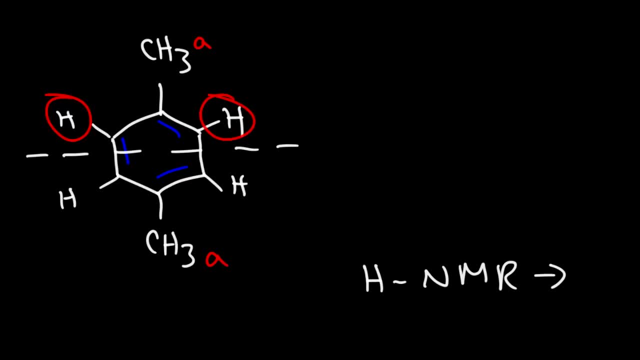 and, at the same time, these two are identical to each other. They're one unit away from the methylglucan, So we're going to work on para-xylene as an example, And we're going to focus on these two. And these two are also one unit away from this methyl group. So all four of those. 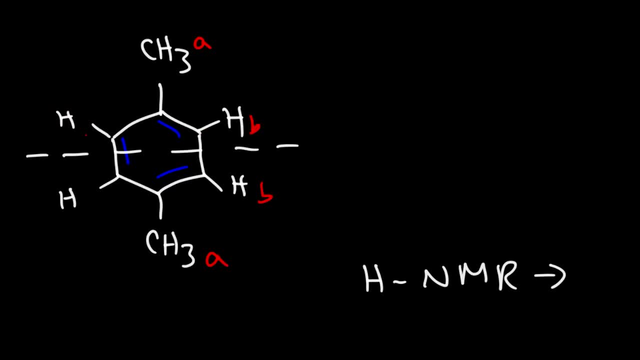 hydrogen atoms are identical to each other. They show up as one signal. So thus we have a total of two different signals in the H NMR spectrum. Now for C NMR, I'm going to use the color green. These two will show up as one signal. Now, these four carbon atoms: they're identical to each other. 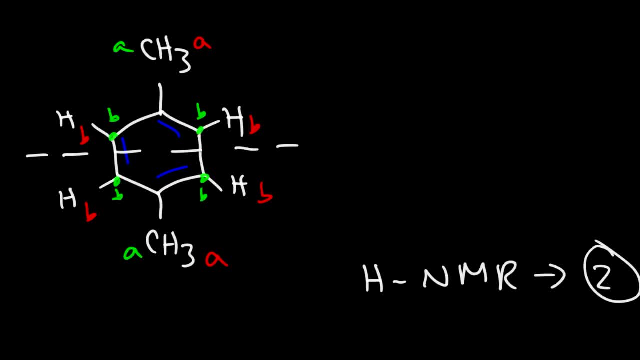 So that's going to be signal B. Now these two carbon atoms which do not have hydrogen atoms. they are identical to each other. So for C? NMR we're going to have three signals as opposed to two. Now let's try ethylbenzene for the next example. 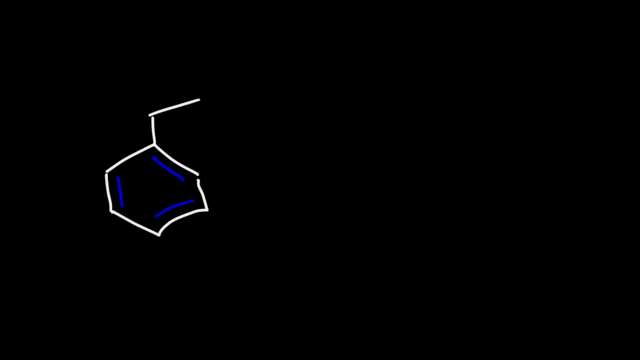 Go ahead and work on that example. So let's try ethylbenzene for the next example. So let's try ethylbenzene for the next example. So let's try ethylbenzene for the next example. 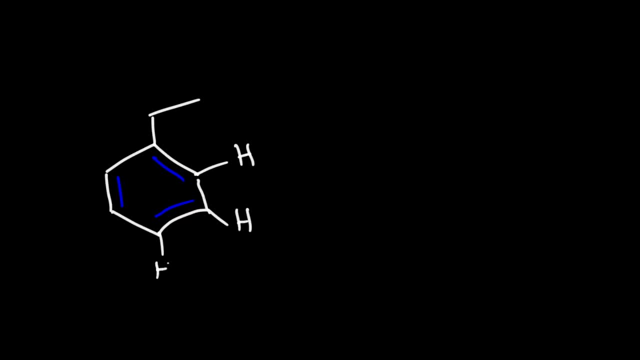 Let's draw the hydrogen atoms Now on the ring. the line of symmetry will be right in the middle. So these two hydrogen atoms are identical to each other. These two are identical to each other, but they're different from this one. These are not the same because hydrogen A is one unit away from the ethyl group, but 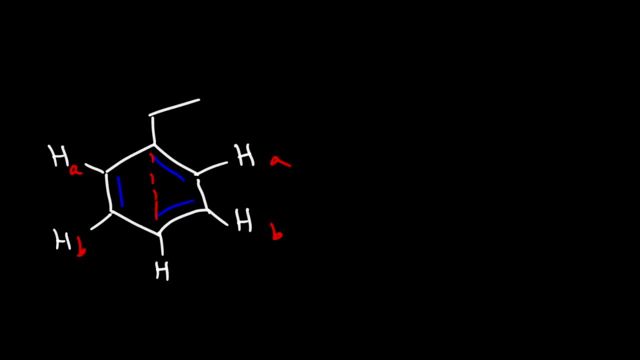 hydrogen B is about two units away from it. This we can call hydrogen C and D and E, because we do have hydrogen atoms on these two carbon atoms. So in the HNMR spectrum we should have a total of five signals. Now for CNMR everything is going to be the same, but we do have this carbon atom that. 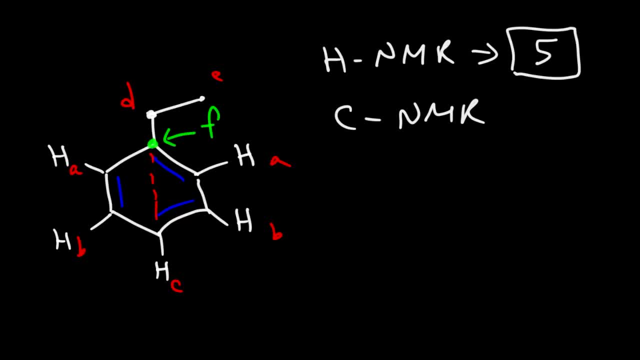 doesn't have a hydrogen atom, So that will Excuse me. That will correspond to signal F in the CNMR spectrum. So we should have a total of six for CNMR. Now what about this one, Meta? dichlorobenzene. 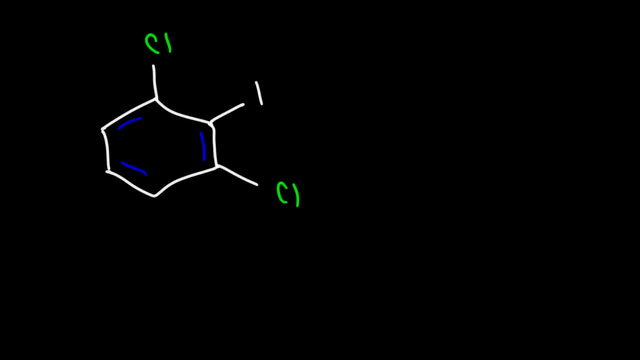 Try that. So let's begin by drawing the hydrogen atoms. Okay, So let's draw the hydrogen atoms. So this is HNMR. Now where is the line of symmetry? I would say the line of symmetry is here, between the two chlorine atoms. 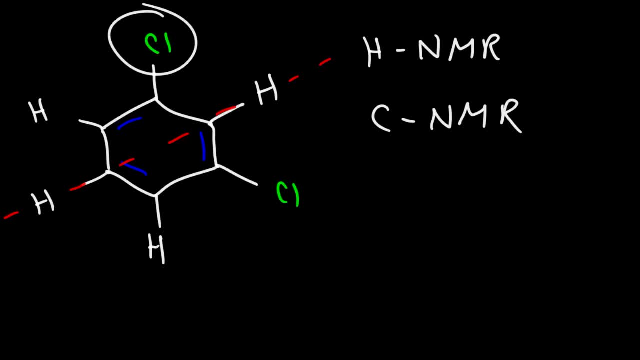 And we could see that these are identical. They're symmetric across the line of symmetry. So this is going to be signal A for HNMR, HNMR, these two signal B, and then this one is going to be signal C. 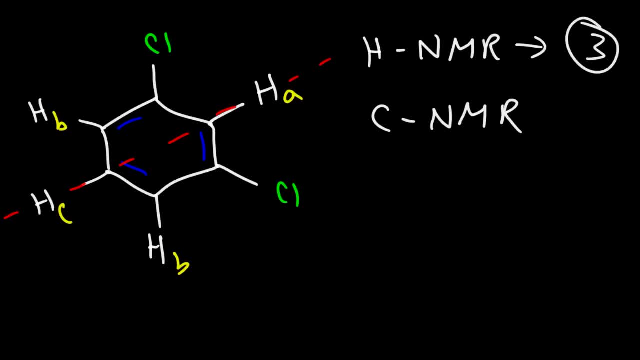 So we should expect three signals in the HNMR spectrum. Now for CNMR, let's use a different color. We'll focus on the carbon atoms, so that's going to be signal A. Here we're going to have signal B, and then for these two carbon atoms that's going to be signal C and for this one D. 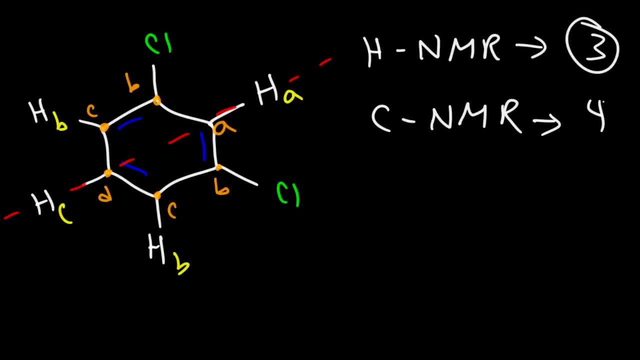 So for CNMR it's going to be one more than HNMR, due to these two carbon atoms, which don't have hydrogen atoms on it. Now let's work on a different example, one that doesn't involve benzene rings. 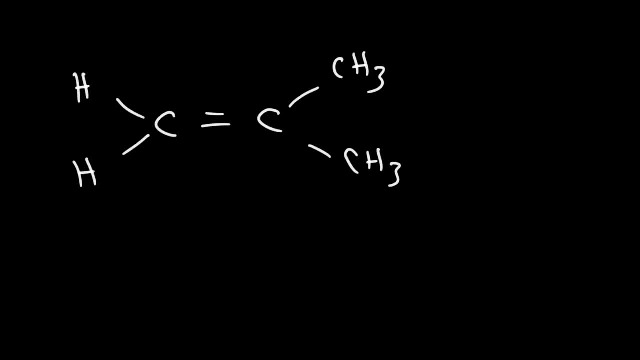 So how many different signals should we expect in the HNMR spectrum for that molecule? What would you say? So these two methyl groups are they identical? Now remember, if you have a carbon-carbon double bond, there's no free rotation. 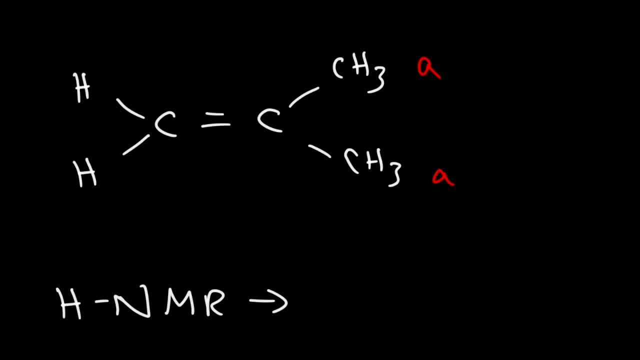 So those two methyl groups are identical. They have the same exact chemical environment. This methyl group here is cis to a hydrogen atom and it's also trans to a hydrogen atom And it's attached to a carbon that has a methyl group. The same situation applies to this one. 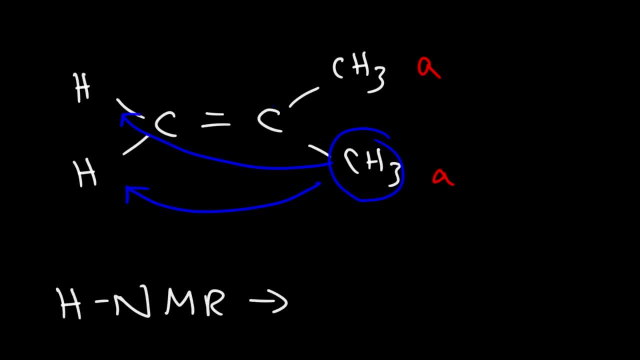 It's cis to this, hydrogen trans to that one and it's attached to a carbon with another methyl group. So they have the same chemical environment. Now, these two hydrogen atoms, they also share the same chemical environment. So that will be signal B. 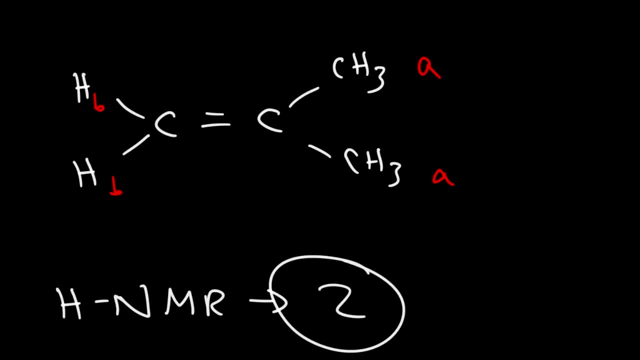 So thus we should get two signals for this particular molecule. How many signals will there be for this molecule? So we only need to focus on these two hydrogen atoms. Are they identical or are they different? So this hydrogen is cis to a chlorine atom and it's trans to a hydrogen atom. 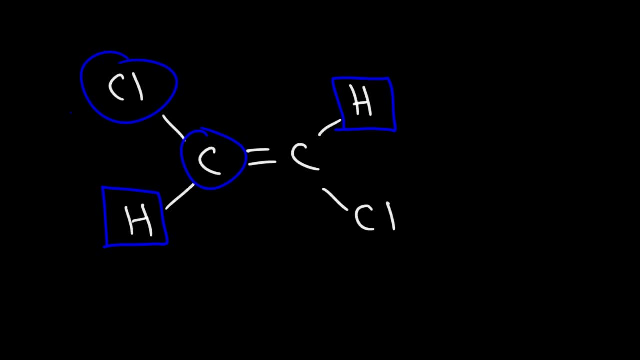 and it's attached to a carbon atom with another chlorine atom. The same is true for the other two. So this is a cis to a chlorine atom. It's cis to that chlorine atom trans to a hydrogen and it's attached to a carbon with a chlorine atom. 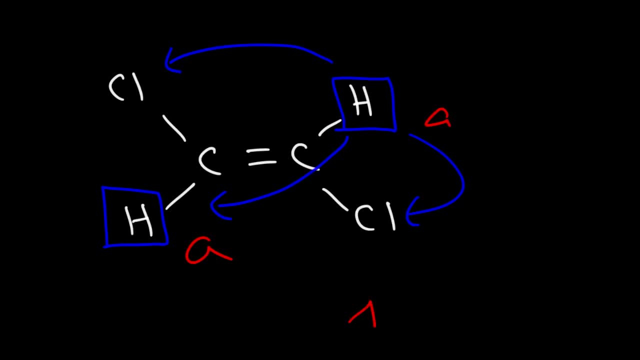 So therefore they're identical. Thus we're only going to have one signal for that molecule. Now let's try one more example. How many different signals should we get for this molecule? How many different signals should we get in the HMR spectrum for this molecule? 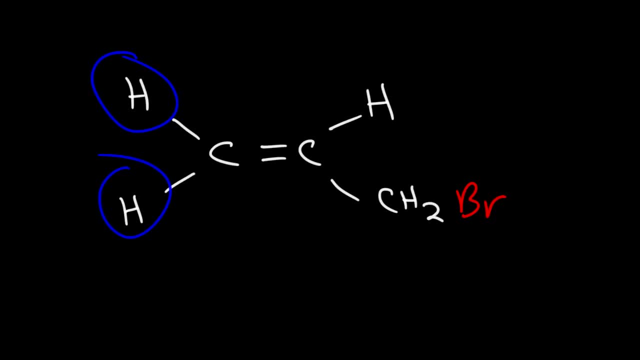 So let's compare these two hydrogen atoms first. Are they identical or are they different? Now, this hydrogen is cis to the CH2Br group, This one is trans to it, So automatically they're different from each other. Now, this hydrogen is going to be different from any one of these two. 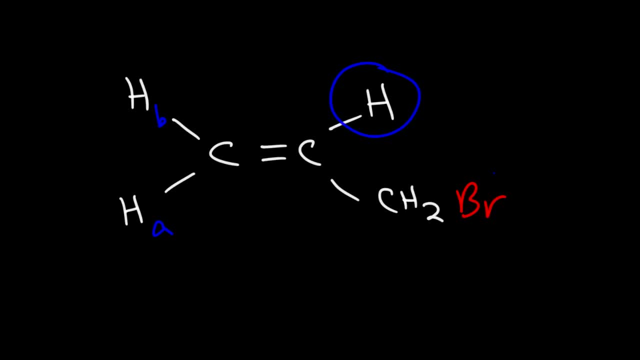 because it's on a different carbon. It's on the same carbon as this group, whereas these two hydrogen atoms are on a different carbon than this group. So automatically, this is going to be a different hydrogen atom. Now, these two hydrogen atoms are different from the rest. 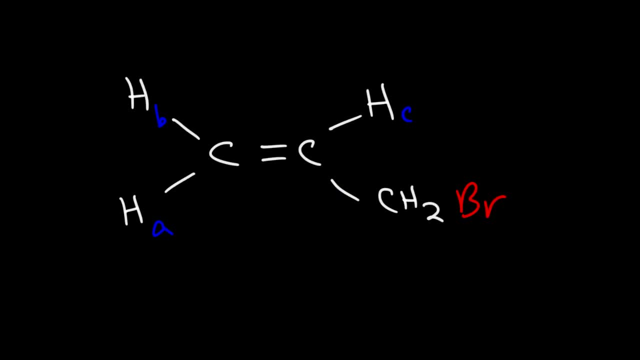 because they are attached to a carbon atom that is directly connected to the bromine atom, whereas all of the other hydrogen atoms are attached to a carbon that does not contain a bromine atom. So this will be signal D. Thus for HNMR we should expect four different signals.